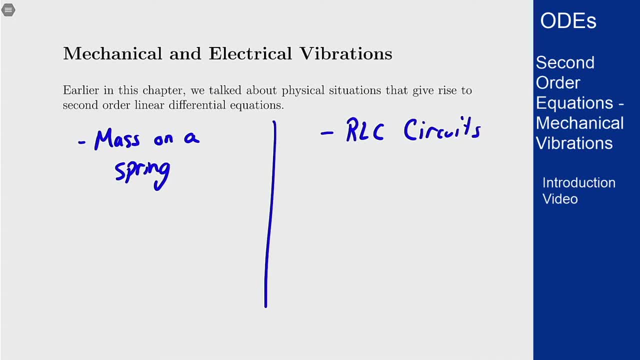 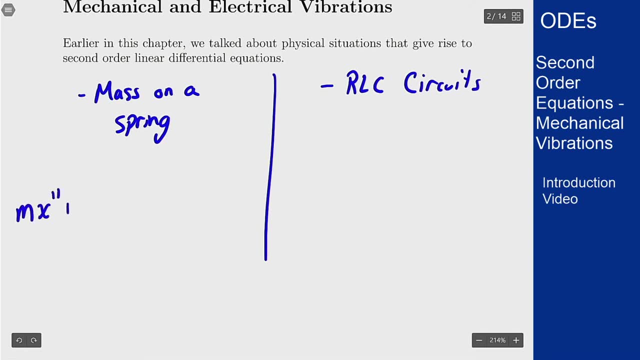 RLC circuits And both of these, if we write them out, give rise to equations that look very similar. For the mass on a spring mass times, second derivative plus drag coefficient or damping coefficient times the first derivative plus spring constant times, the function. 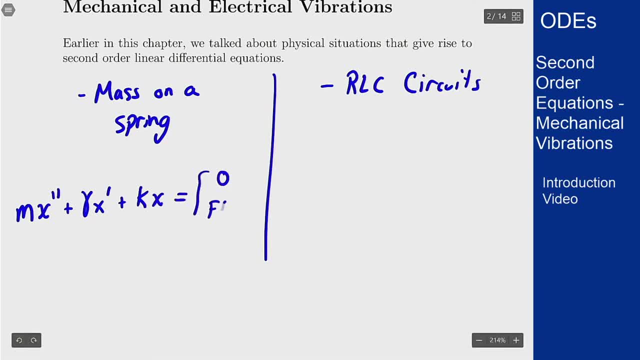 equals zero or some function, depending on if there's extra forces going on. And for circuits we get a similar setup: The inductance, second derivative of the charge, plus the resistance times the first derivative Plus one over the capacitance times. the charge itself equals either zero or some voltage. 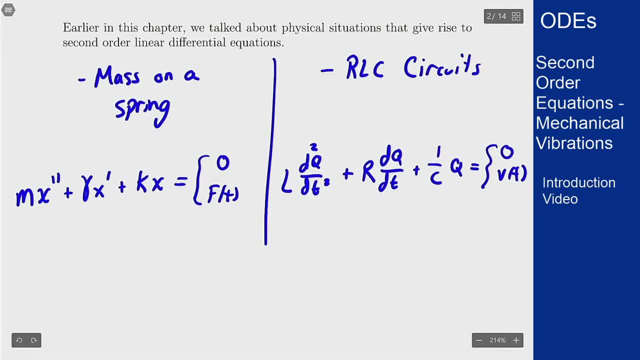 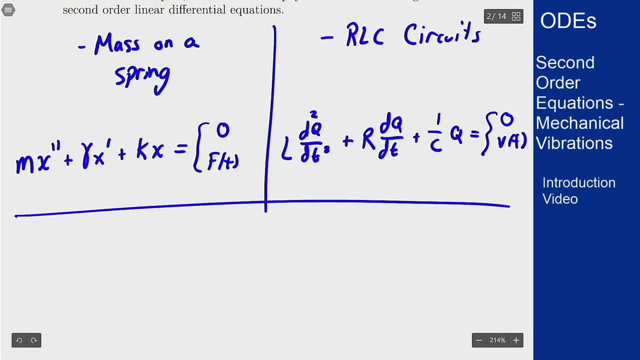 applied to the circuit. So in either case, here we're down to a second order constant coefficient equation. So we're left with something like a times y, double prime plus b, times y prime plus c, times y equals f of t, And we're left with a function that's going to be zero, depending on the situation. 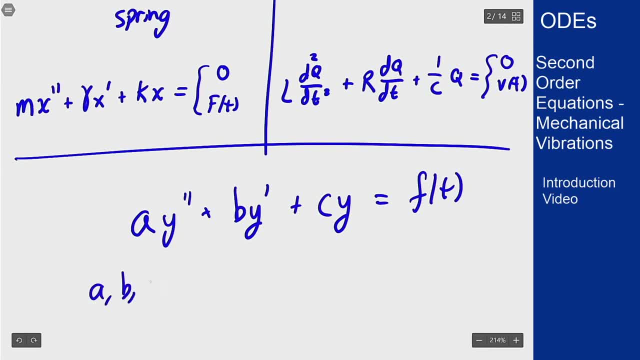 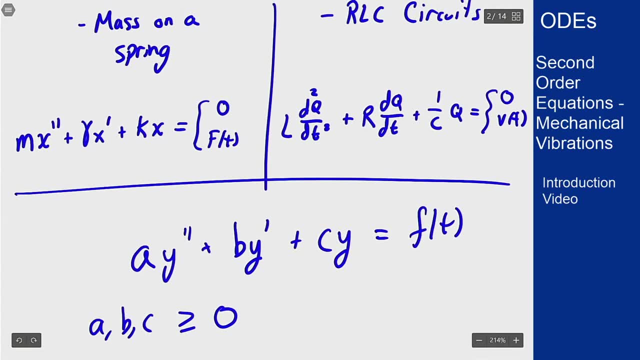 And in this case we're assuming here that a, b and c are all are at least positive numbers. So if we think about the physical systems we get to equations like this. we can abstract that into this sort of a system here. 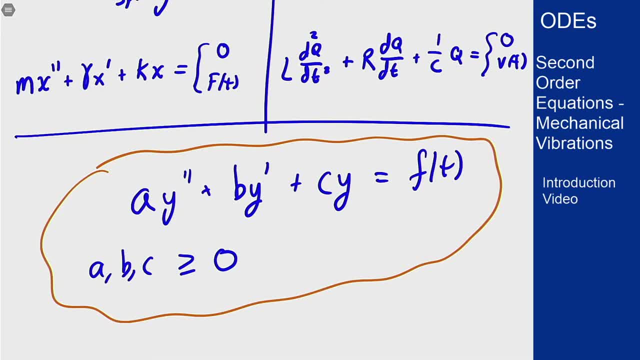 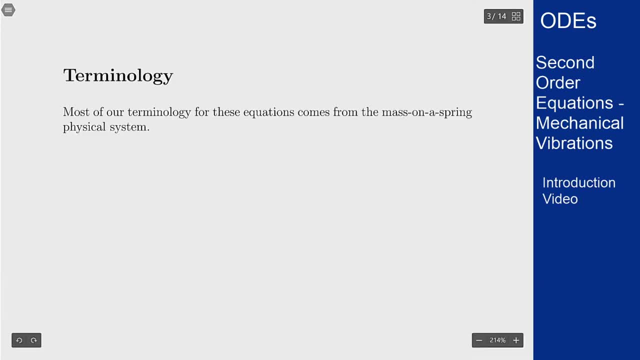 And these know how to solve, at least for when the function on the right side is zero. We'll focus here on the case where this is zero and deal with the other part later on. So our terminology that we use for these equations a lot of times comes from this: 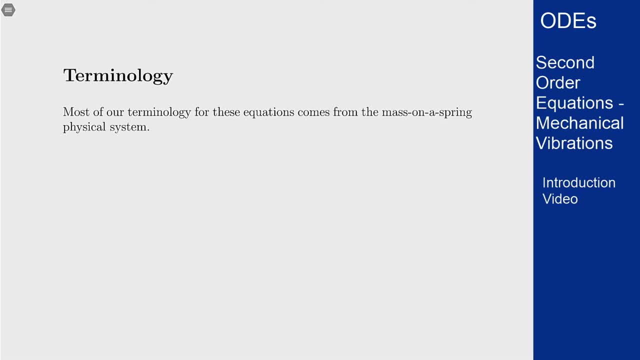 mass on the spring system. So you think about the physical system and the words used to describe that are related to the differential equation that models it. If we go back to our model, which was a- y double prime plus b, y prime plus c, y equals zero or a function f of t, we say that: 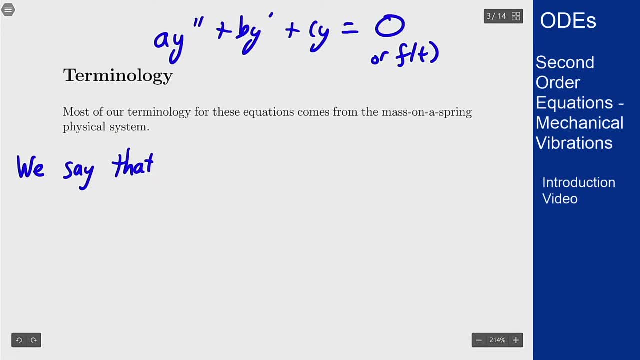 the equation is unforced or free, if the right hand side is zero, That is, if the equation is homogeneous, Which basically comes from the idea that unforced means there's no extra forcing applied, There's no external forces outside of just the acceleration, the drag and the spring. 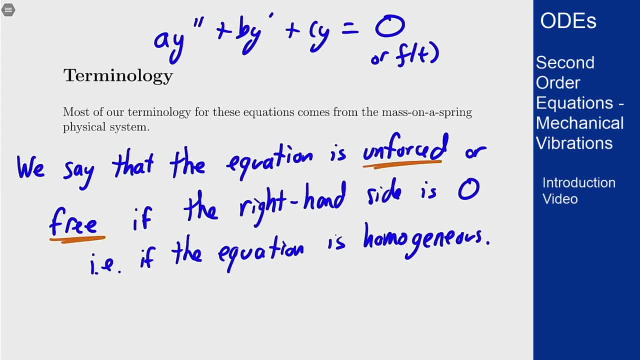 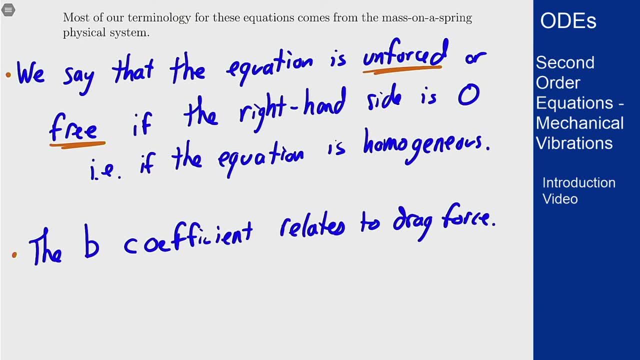 constant. If there's no other forces, we say it's unforced or a free system. The B coefficient here relates to drag force, or how much the system is impacted by its external environment in terms of restricting the motion of this object. This is called the damping coefficient because it sort 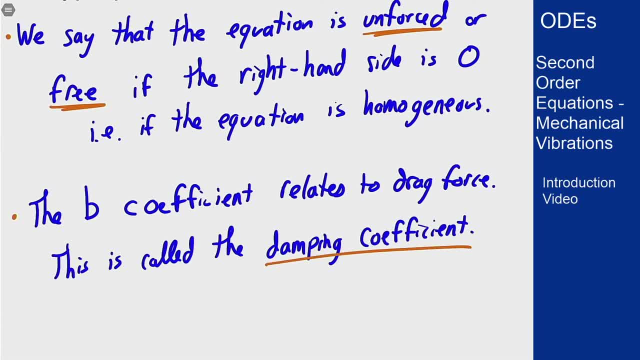 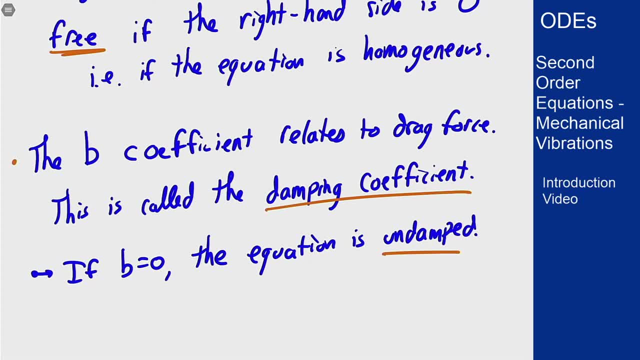 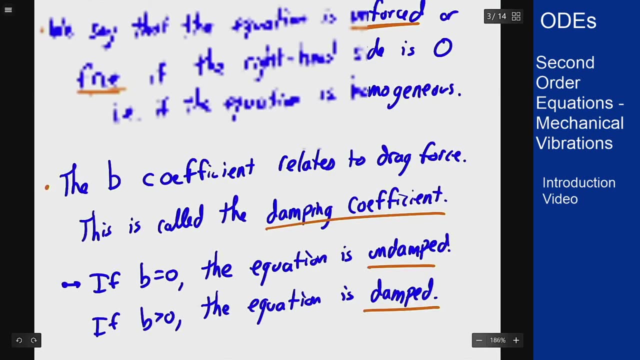 of dampens, the oscillation of the movement by controlling how it can behave If B is zero. you see the equation is undamped. Otherwise we say it is a damped equation. We'll have different conditions on this damped equation that we'll see here in a second. So these words about being unforced or free equation or a, 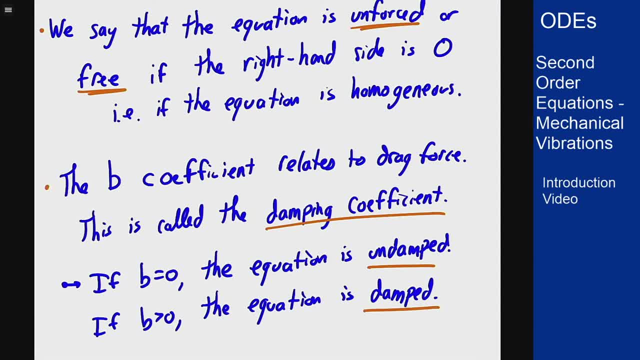 forced equation, which is the opposite of that, comes from whether it's homogeneous or not, and we have the damping coefficient, that is, this B of this derivative term in the middle. Now, as long as this equation is homogeneous, we know how to solve it. If it's constant coefficient, 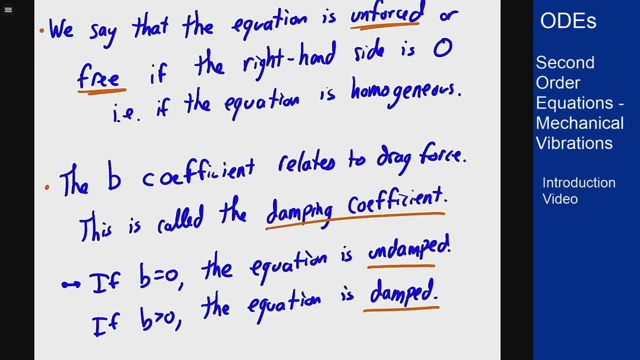 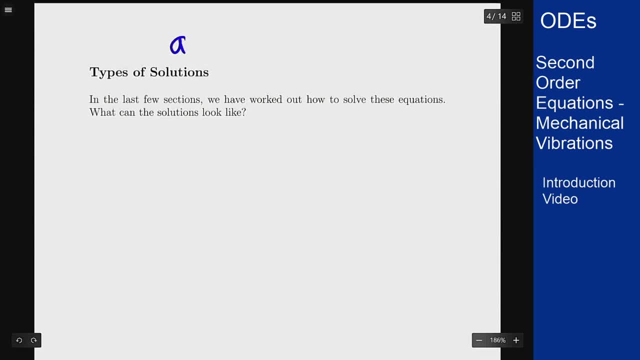 it's second order, it's linear, it's homogeneous. we know how to solve all of those problems about the methods we've discussed previously, So we can handle them. So we have our main equation again and there's different types of solutions you can get based on values of A, B and C. So, for instance, if we have B equals zero. 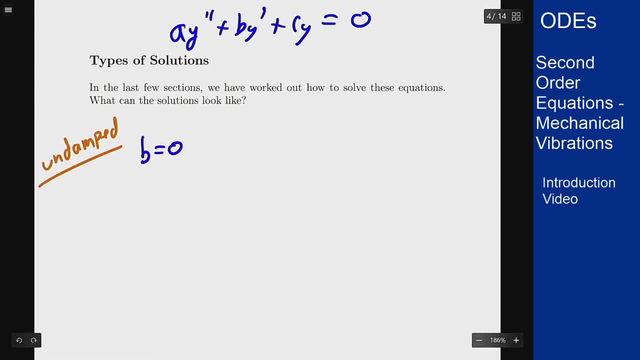 this is our undamped equation. In that case, what do we get? Well, our equation is: A- Y, double prime plus C. Y equals zero. If A and C are both positive, these will turn into pure sine and cosine equations. If A and C are both positive, these will turn into pure sine and cosine equations. 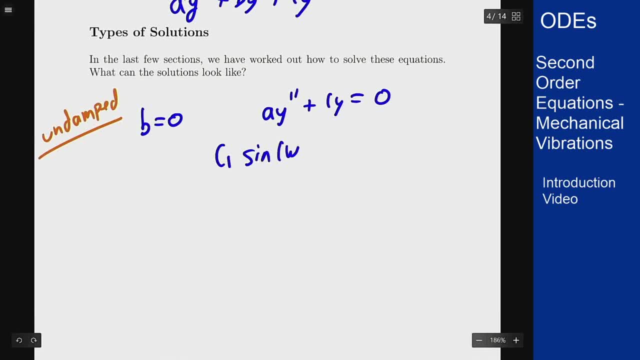 So we'll end up with a C1 sine of omega t plus a C2 cosine of omega t. This is sort of a free oscillation, and this is the idea why these are called vibrations, because if we draw this out right, this is a function that will just oscillate up and down forever, hence a vibration. Now what? 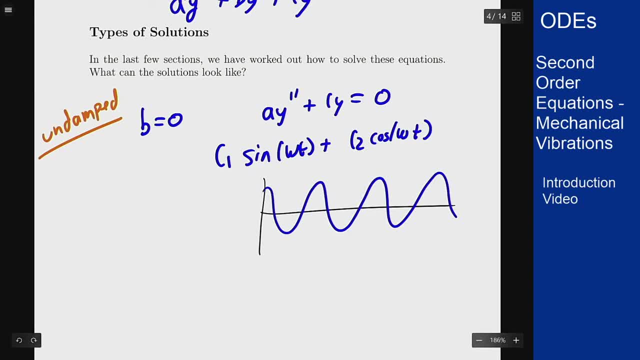 happens if B is a little bigger than zero, but not very much. Well, in that case we'll have that B squared minus four. A C is less than zero, So we'll have that B squared minus four. A C is less than zero, So we'll have that B squared minus four. A C is less than zero, So we'll have that B squared minus. 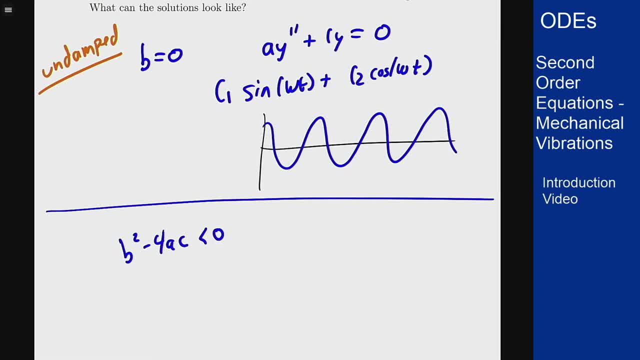 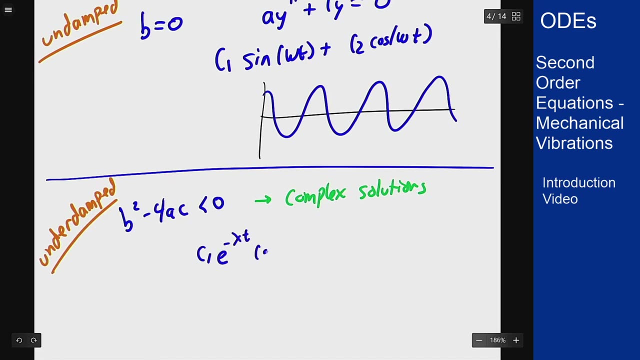 four B is less than zero, So we'll have that B squared minus four A C is less than zero, So we'll have like a C1e to the minus lambda t cosine of u t positive. moins happens to be positive, but this shouldn't happen. Plus sign for sin. 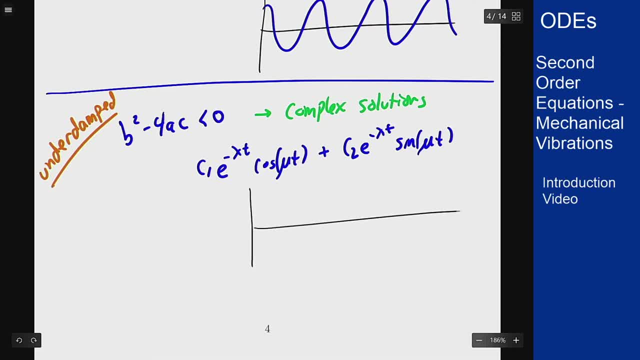 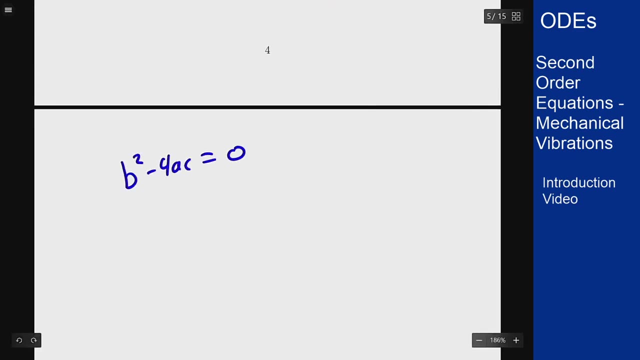 And this is the same idea, but they're going to decay in time. If it oscillates, but not periodically, because it's going to decay to zero in time. We have two more options here We have. if b squared minus 4ac equals zero, This is the critically damped case. In this case, our solution is the. 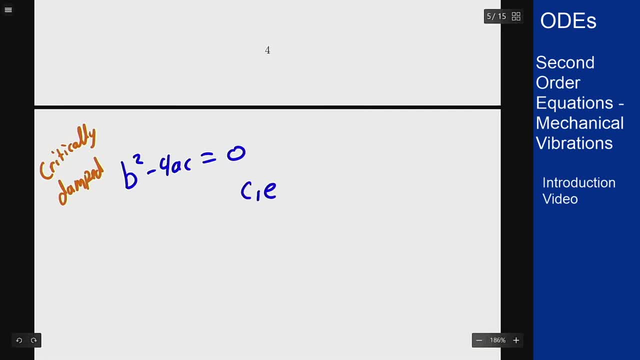 double root solution. So we're going to get a c1 e to the rt plus a c2 t e to the rt, and that gives us decay to zero or potentially one oscillation and decay to zero. This does not oscillate, it just goes sort of straight to the equilibrium point or passes through zero once And the last. 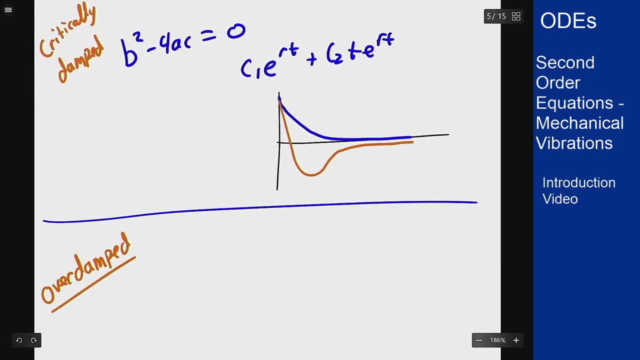 case is what we call overdamped, and this is when b is really big. So when I have b squared minus 4ac, bigger than zero, I'm going to get two real roots. So in this case I get sort of a, c1, e to the r1 t. 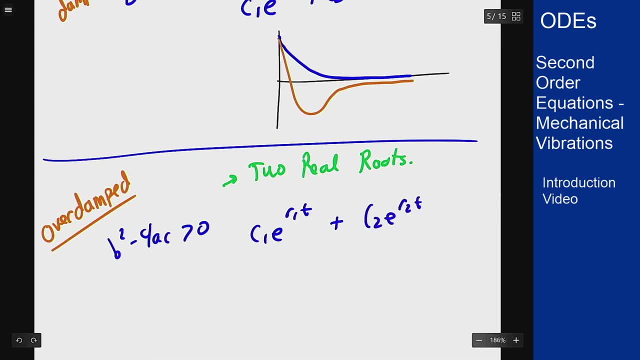 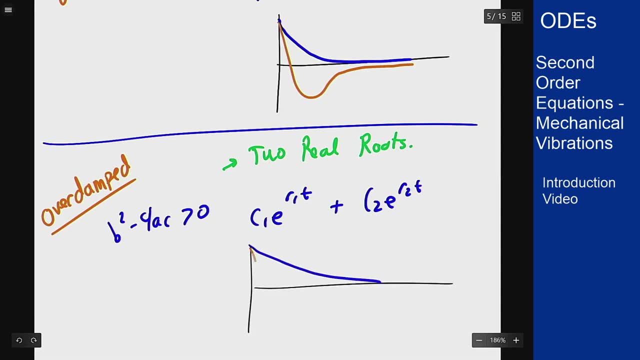 e to e to the r2. t. R1 and R2 are both negative here. So what I end up with is decay. Same sort of idea, either decay or one oscillation and decay, But in general this decay is going to be slower than the critically. 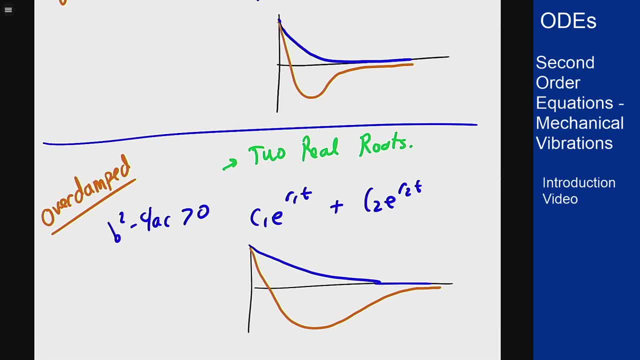 damped case. There's all different words to talk about these solutions. We could talk about them being undamped, under damped, critically damped or overdamped. based on these parameters, You get an idea for how these solutions behave based on these different properties. If you want to know, 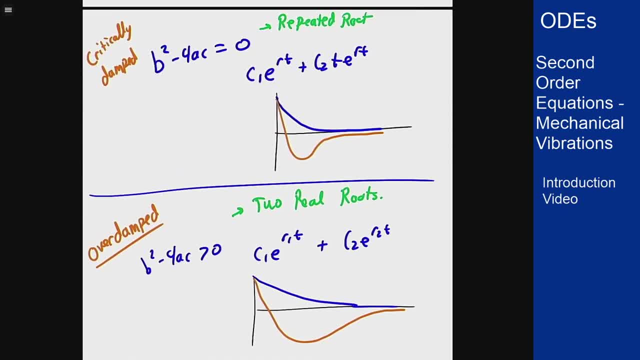 both what these words mean, how they relate to each other and how they're related to each other, to the equation, and how they relate to the different types of resolution. it can be on, given that it meets those different properties.